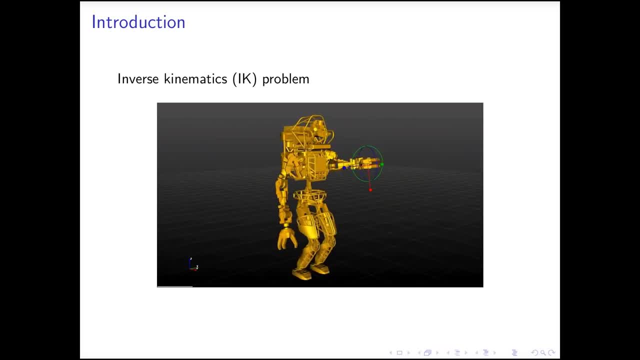 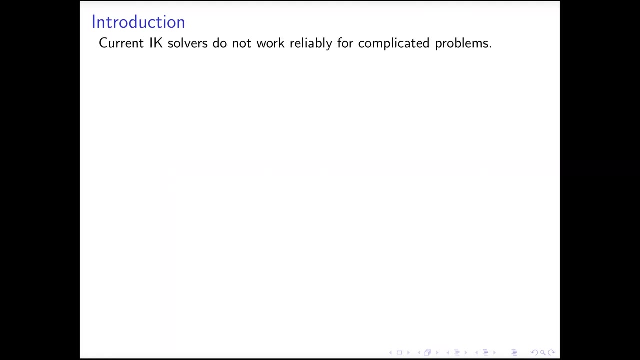 Inverse kinematics is one of the most fundamental problems in robotics In the era of deep learning and robot doing backflipping. you may wonder why I am interested in this fundamental problem. Well, to me, most IK solvers do not always work very reliably, especially for complicated problems. 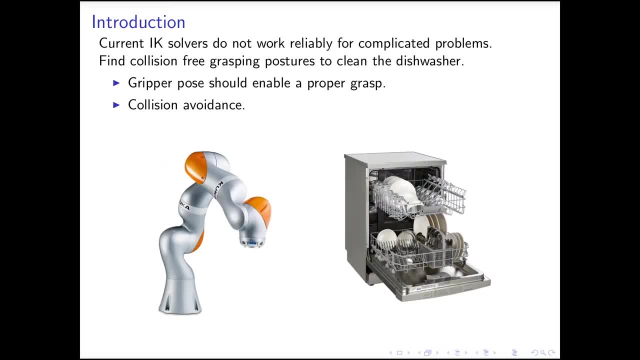 For example, if we want to use this robot arm to clean the dishwasher, we might impose a constraint: that the robot hand should not reach the center of mass above the foot support region. In this case, we think that a gripper pose should enable a proper grasp. 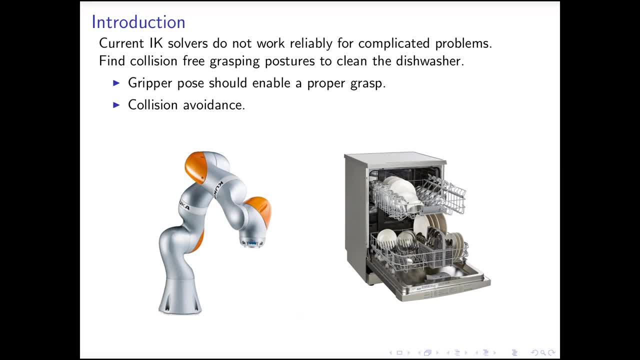 So instead of specifying one single desired gripper pose, there is a whole set of possible gripper poses. Also, we want our posture to be collision-free. This can be a challenging problem to many IK solvers, as they cannot guarantee to solve the problem 100% of time. 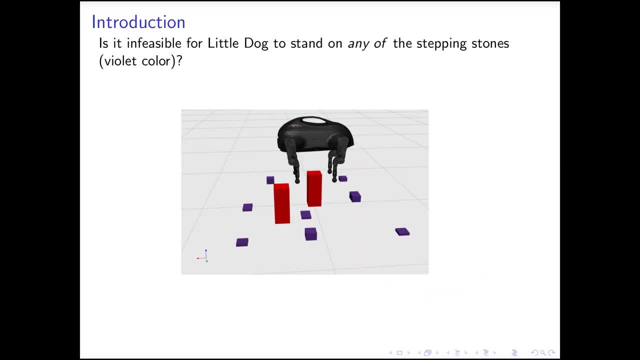 Here is another example. We ask: is it infeasible for the little dog to stand on this step? Most IK solvers cannot answer this question because, first, they do not certify global infeasibility and, second, the solver needs to assign each leg to one of the stepping stones. 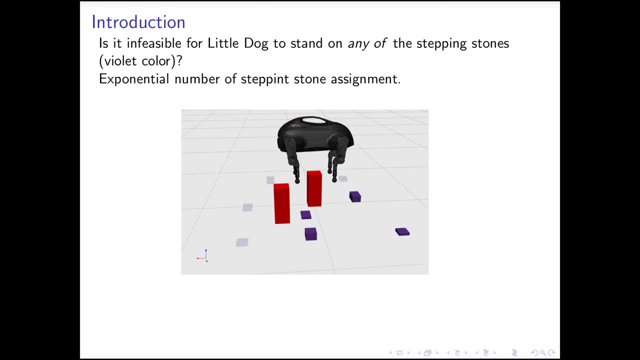 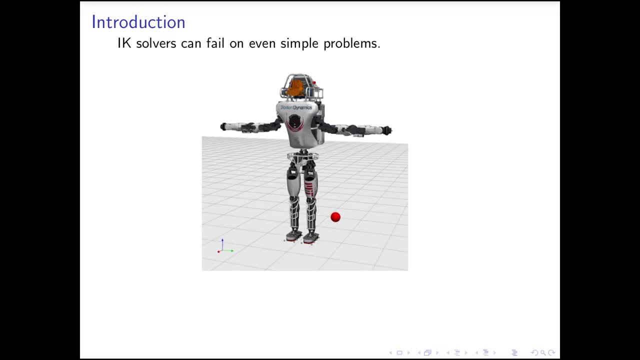 There are exponential number of stepping stone assignments, and it takes too long for the solver to enumerate all combinations. Moreover, the IK solvers can fail on even simple problems. Here we want the robot hand to stand on this step. Here we want the robot hand to reach that red sphere. 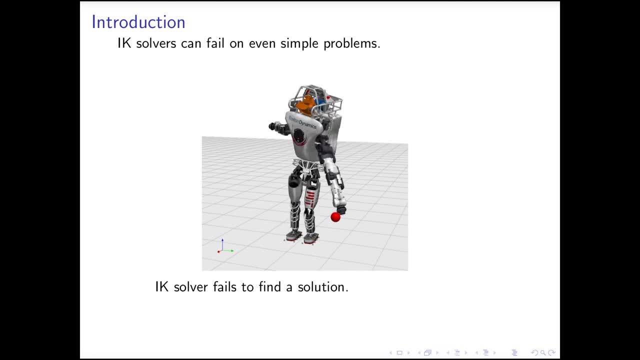 The IK solver fails. This is the best solution it finds, But that red sphere is reachable. The IK solver fails because it only searches within a local neighborhood of the initial guess, while the solution is far away and the initial guess is singular. 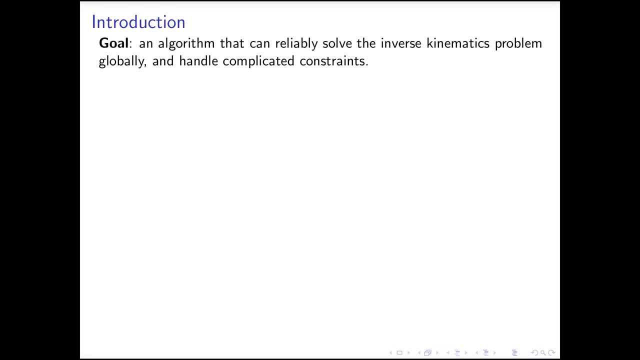 To remedy all these problems. we want to come up with an algorithm that can solve the inverse kinematics problem reliably, Even for complicated constraints. By reliably I mean first when the IK problem is feasible, then the algorithm can always find a solution. 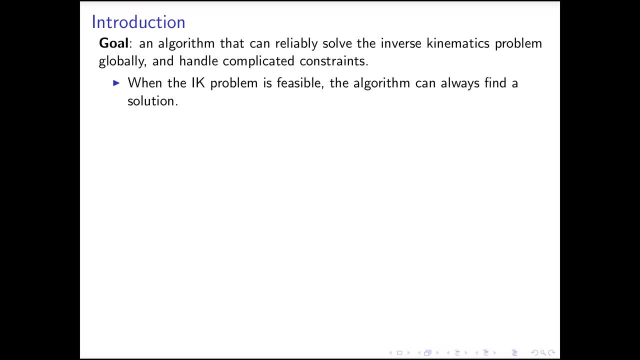 On the other hand, when the algorithm cannot find a solution, it proves that the IK problem is globally infeasible. Here we show some results by running our algorithm. On the left-hand side, I show the collision-free posture for a robot arm to grasp a mug on the clutter table. 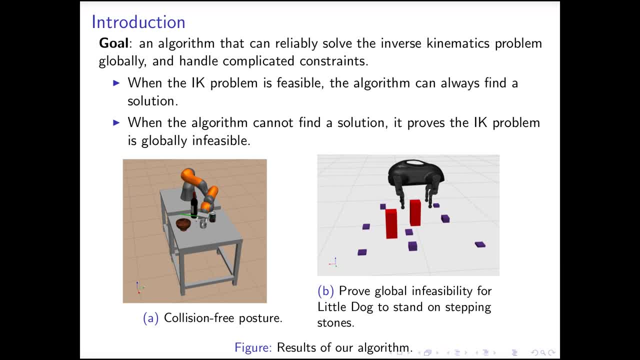 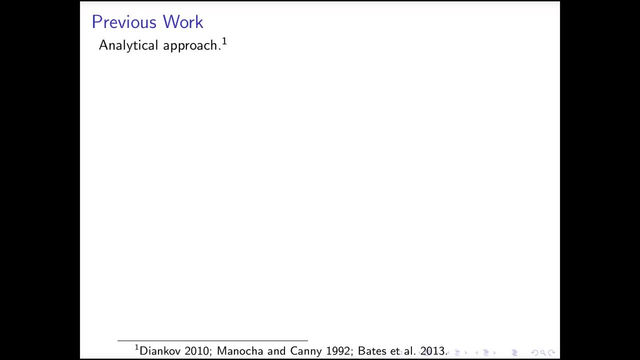 On the right-hand side. our algorithm can prove it is globally infeasible for the little dog to stand on these stepping stones. There has been a lot of research on solving IK problems. First there is the analytical approach that if we only have equality constraints, 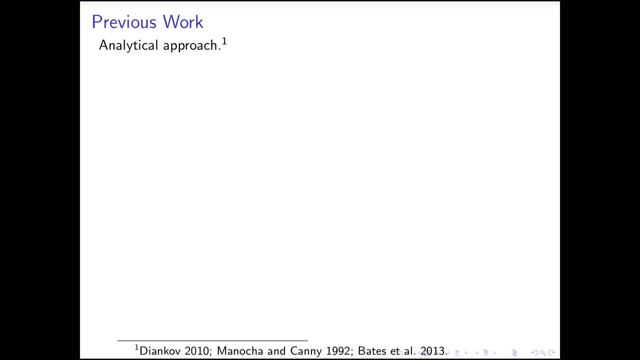 and if the robot structure is simple, then we can solve the IK problem in the closed form. The shortcoming of this approach is that it is not suitable when we have inequality constraints or when the robots are complicated, For example, if we want to find the posture of the little dog. 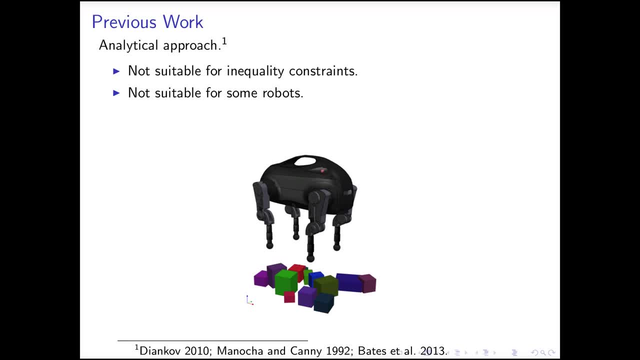 standing on these stepping stones. the region of each stepping stone is described by inequality constraints. Thus analytical approach does not apply. On the other hand, there is the iterative numerical approach, In which it solves the IK problem through gradient-based nonlinear optimization. 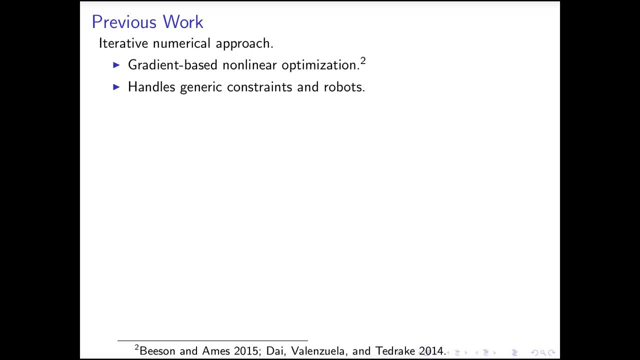 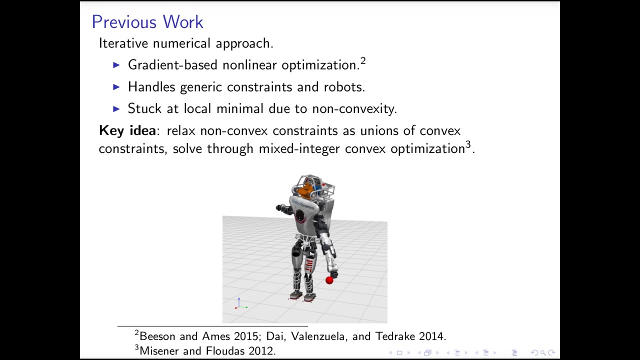 This approach can handle complicated constraints and robots. The shortcoming is that it can get stuck at local minimum due to nonconvexity of the problem. The key idea of this paper is to relax the nonconvex constraints to a union of convex constraints. 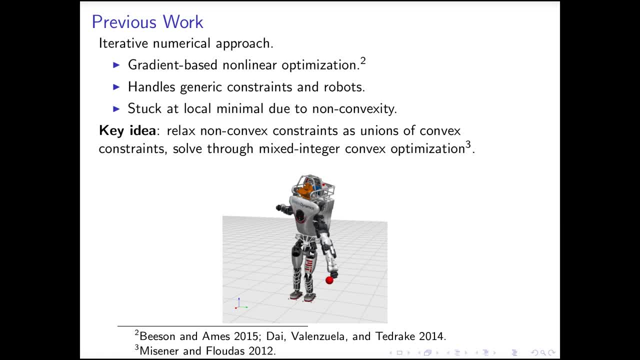 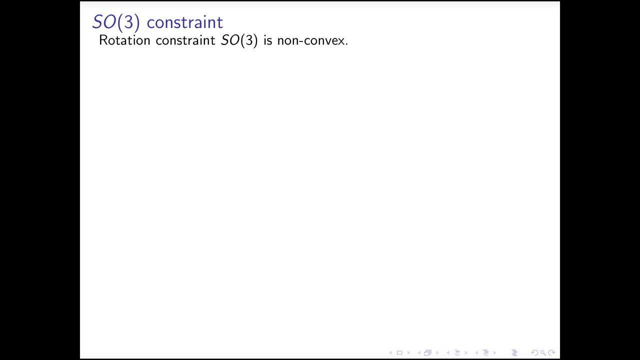 which can be solved by mixed integer convex optimization. In the next few slides I will explain how we shall apply this idea to IK problems. The nonconvexity of IK problem originates from the nonconvex SO constraints, So we will focus on rotation first. 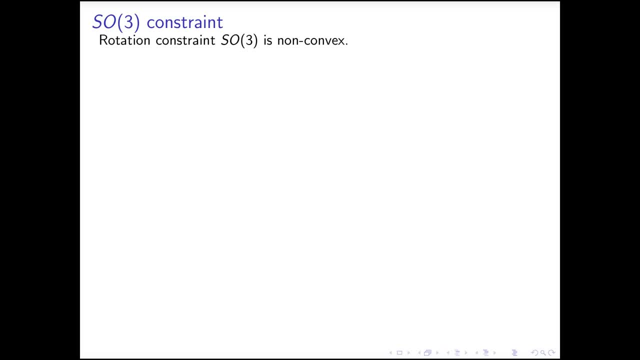 There are several ways to represent a rotation, such as using equinoxes, quaternions, etc. Here we choose the rotation matrix representation, Since the position of a point after rotation is a linear function of the rotation matrix, while it would be nonlinear if we were to choose other representations. 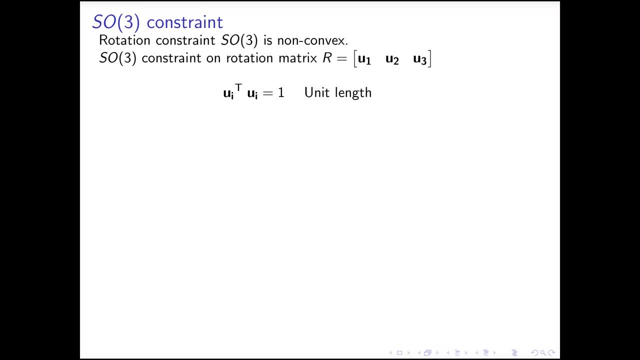 The SO constraints on the rotation matrix include: each of its columns has unit lengths and two columns are orthogonal. Finally, a cross-product constraint to rule out flipping from rotation. It is easy to see that these constraints are nonconvex, For example for the unit length constraint. 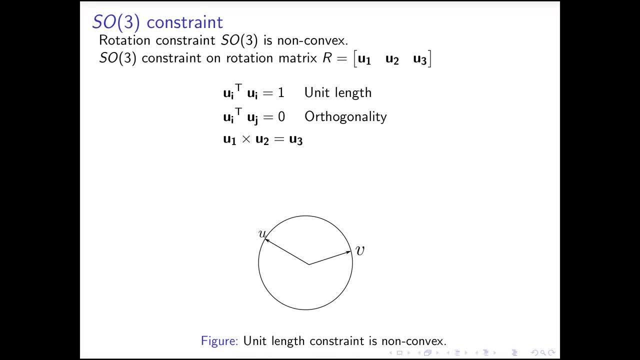 if we take two vectors with unit lengths, their convex combination does not have a unit length. Thus the constraint is nonconvex. We will apply the idea mentioned in the previous slide to relax the nonconvex, SO constraints as unions of convex constraints. 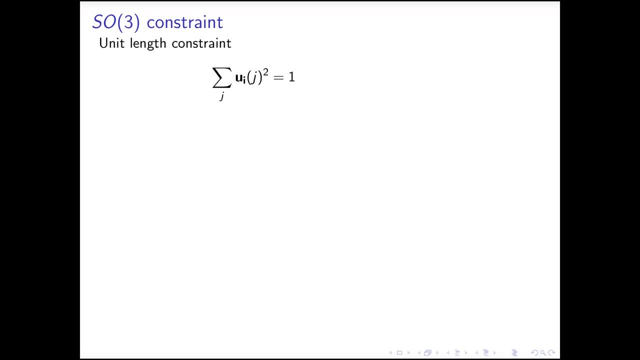 How shall we do that? Let's first look at the unit length constraint, which can be expressed as: the summation of quadratic terms equals to 1.. Here I plot the curve of one quadratic term, Although this curve is nonconvex. 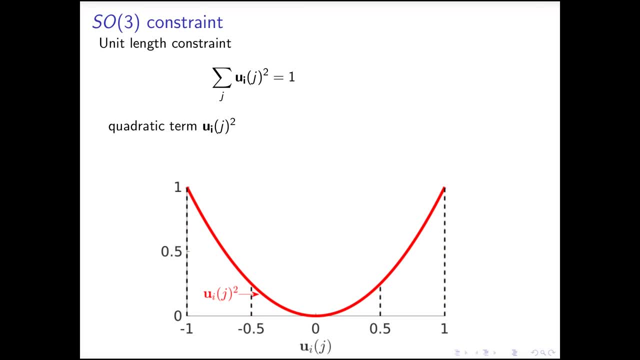 we can cut it into smaller pieces and compute the convex hull of each small piece. We then introduce a slack variable, w, as the approximation of the quadratic term, by requiring that the point w to be within one of the convex hulls. This can be formulated as a mixed integer convex constraint. 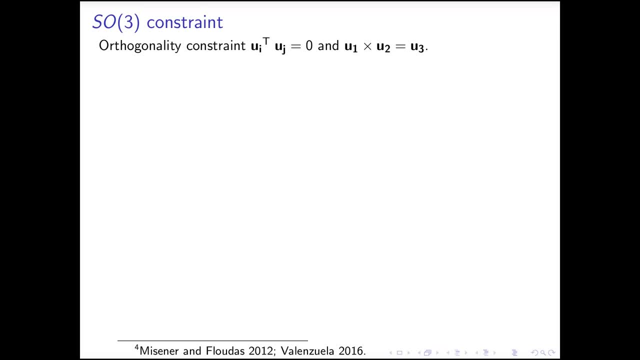 For the orthogonality and cross-product constraints. they can be expressed as the summation of bilinear terms in the form w equals to x times y. Here I plot the surface of the bilinear term- w equals to x times y- from two perspectives. 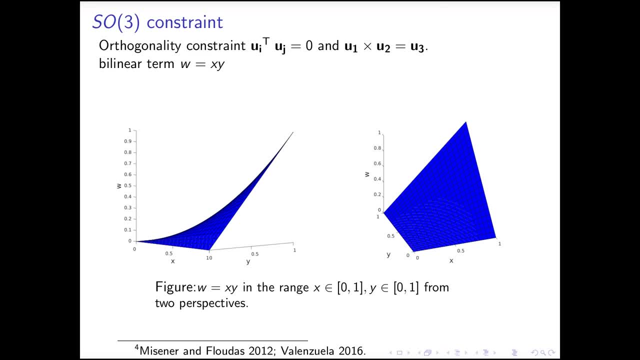 Although this surface is nonconvex, we can compute its convex hull as a relaxation. On the left-hand side, I show the paranormal view of the nonconvex surface together with its convex hull. To obtain better relaxation with higher accuracy, we can cut the original surface into smaller pieces. 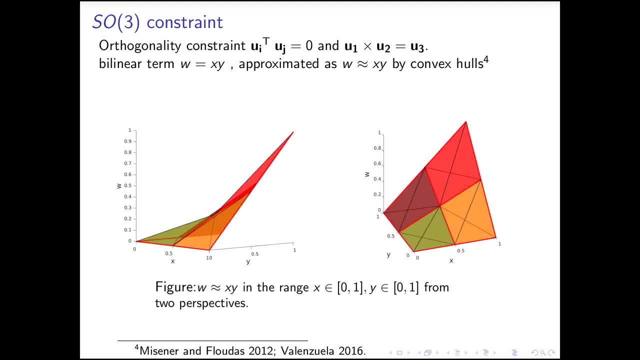 and compute the convex hull of each small piece. On the left-hand side I again show the original surface together with each small convex hull. So we have relaxed the nonconvex SO constraints as unions of convex constraints. How shall we use this SO relaxation? 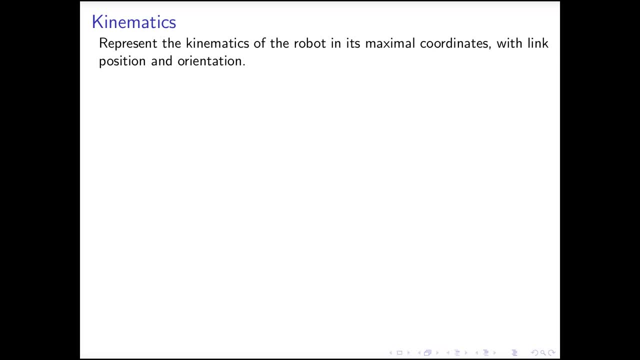 We will represent the kinematics of the robot in its maximal coordinates, with both link position and orientation as decision variables, and require that the link rotation matrix satisfy the SO relaxation. We also need to impose the kinematic constraints that two links are connected together through a joint 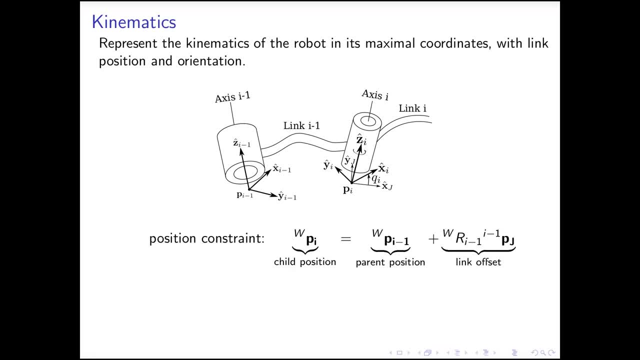 To do so, we impose a position constraint on the child link and an orientation constraint on the axis of the connecting joint. Both constraints are linear with respect to the decision variables. We can handle a rich set of kinematic constraints, including both equality and inequality ones. 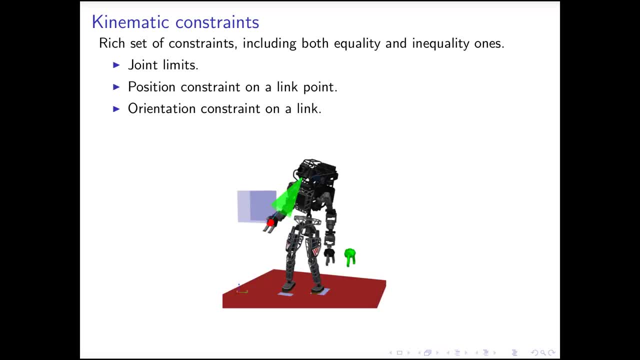 such as joint limits, position constraints, orientation constraints, etc. In the bottom I visualize one scenario of our IK problem: that we want the robot foot to be within some stepping regions. also its right hand to be within a bounding box and its head camera is gazing at its right hand. 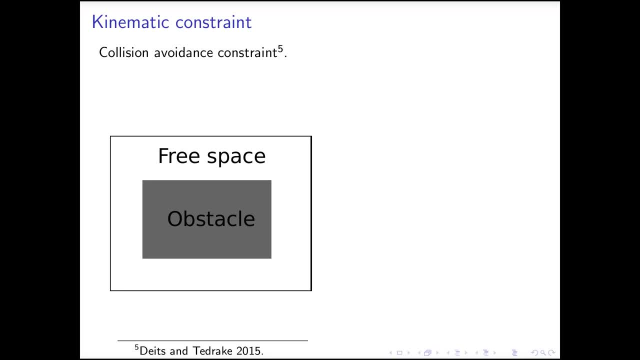 Moreover, we can handle collision avoidance constraints. We do that by representing non-convex collision-free space as a union of convex small regions, as shown below, and require that link points to be within one of the small convex collision-free regions, which again can be formulated. 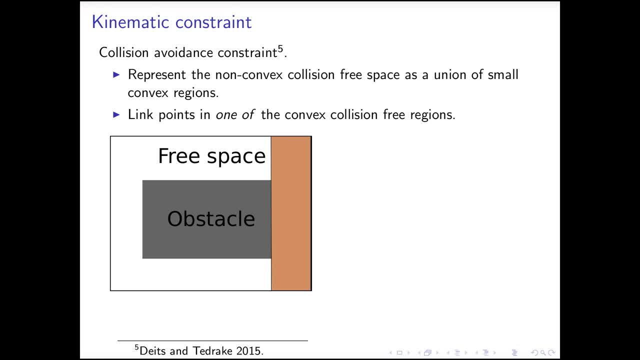 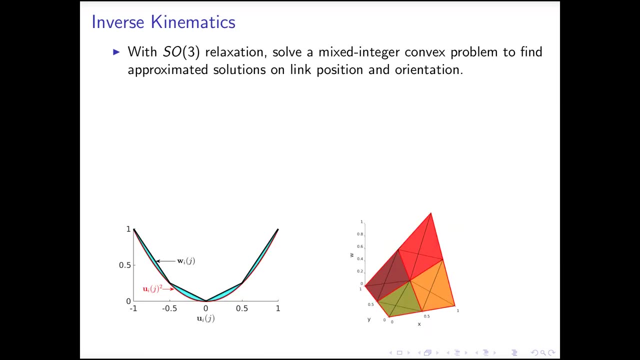 as a mixed integer convex constraint. There are many approaches to segment-free space. On the right hand side we use a naive approach to represent the free space as unions of bounding boxes. Here I quickly summarize our IK algorithm With our SO relaxation: 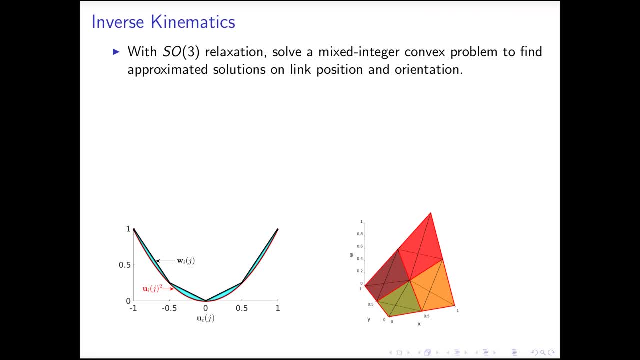 we can solve a mixed integer convex optimization problem to find approximate solutions to link position and orientation. We then project the approximate link rotation matrices back to SO in the closed form to find the joint angles. There are two possible outcomes when solving the mixed integer convex problem. 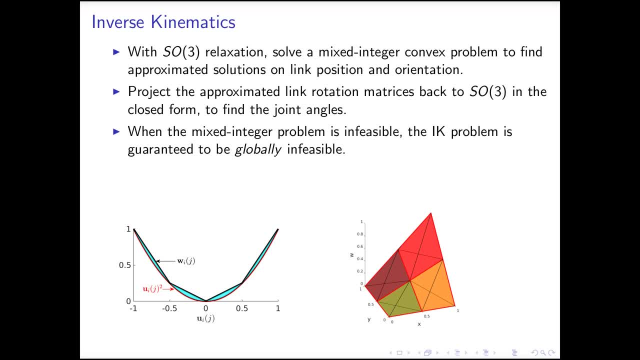 If the optimization is infeasible, then we prove that the IK problem is globally infeasible. If the optimization is feasible, then we find solutions that approximately satisfy the kinematic constraints. We apply our algorithm on a 7-DoF robot arm. 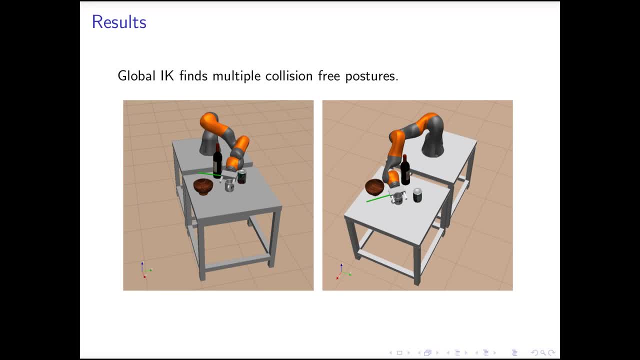 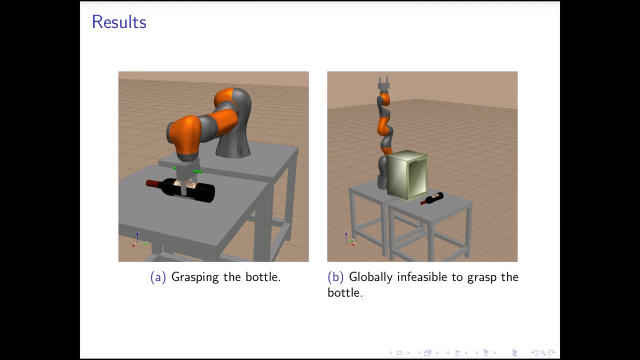 to find collision-free postures such that the arm can grasp the mug on the cluttered table. Since we solve the IK problem globally, our approach finds multiple collision-free postures instead of a single one. Our approach can also detect infeasibility. 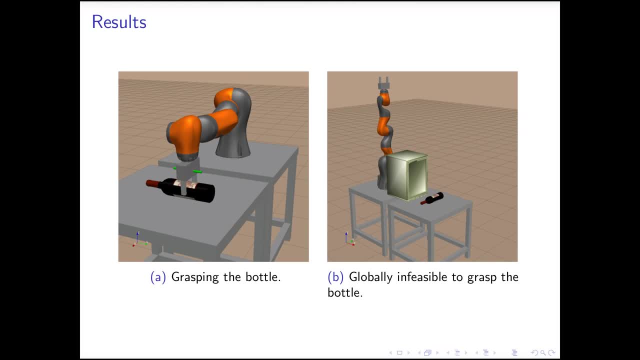 On the left hand side, our solver finds a poster for the arm to grasp a wine bottle on the table On the right hand side. if we put a wine fridge in between the arm and the bottle, then our approach proves that it is globally infeasible. 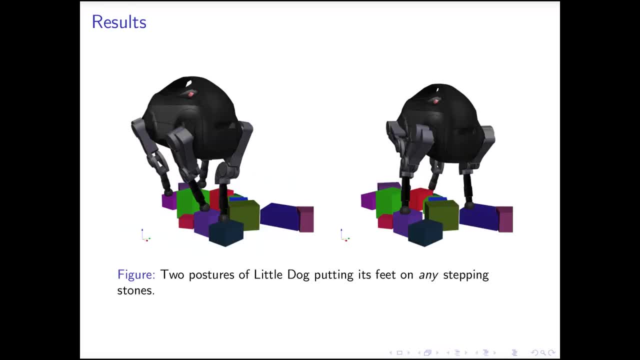 to find a grasping poster. We also apply our approach to the little dog. It finds multiple postures for the robot to stand on different sets of stepping stones. This demonstrates that we can search over all possible stepping stone combinations simultaneously. We put the stepping stones farther away. 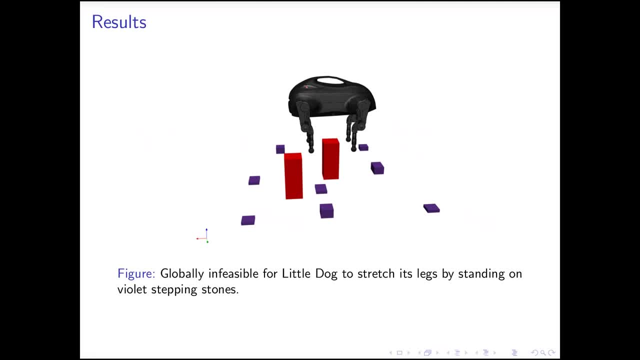 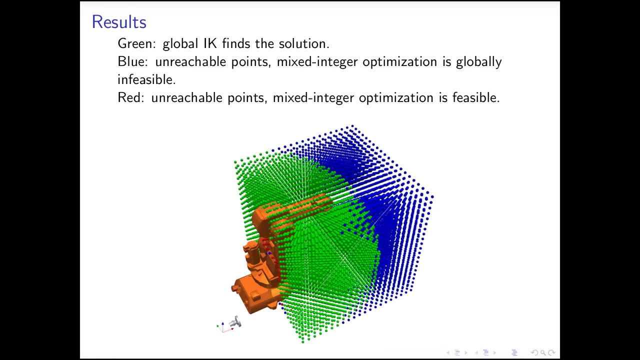 and our approach proves it is globally infeasible for the little dog to stretch its legs so that it can put each of its feet on one stepping stone. Our approach proves the infeasibility of all combinations simultaneously. Finally, we test our approach more thoroughly. 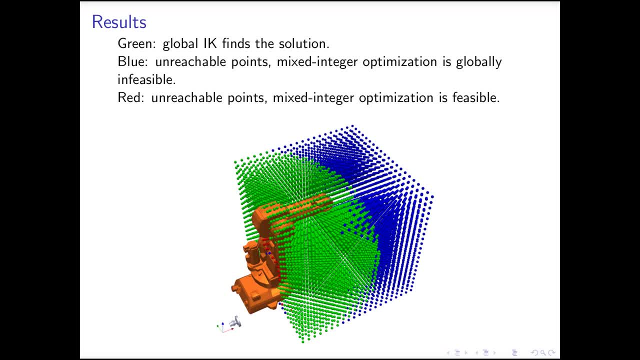 on a six-stove robot arm, We require that the ND factor of the arm to reach each sampled point with the orientation shown in the bottom left. This IK problem can also be solved analytically and we compare our results with the analytical results. 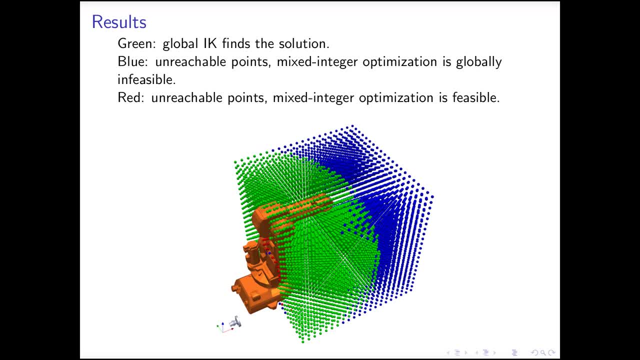 For the green and blue dots, our approach agrees with the analytical approach that they both think that the point is either reachable or unreachable. There are also some red points which are actually unreachable, but our mixed integer optimization is feasible. This is because our approach